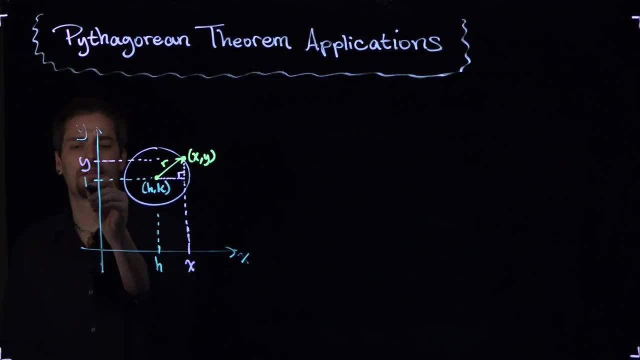 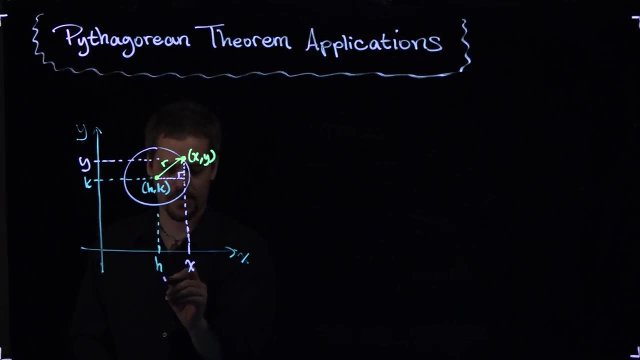 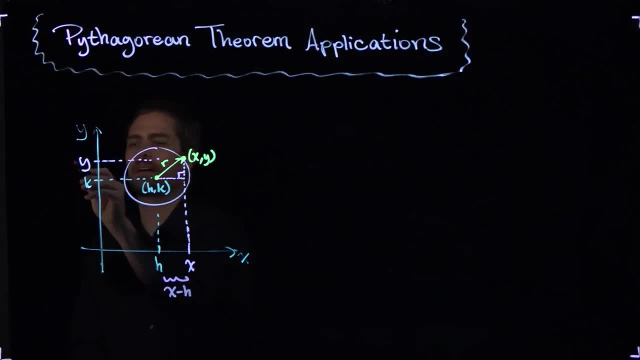 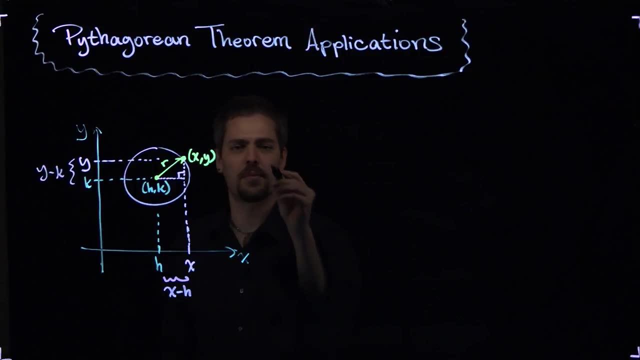 here is x minus h and this little distance up here is y minus k. So when I stick that into the theorem I can say: oh, this distance, x minus h, quantity squared plus this little piece of a distance. So y minus k, quantity squared must be equal to r squared. 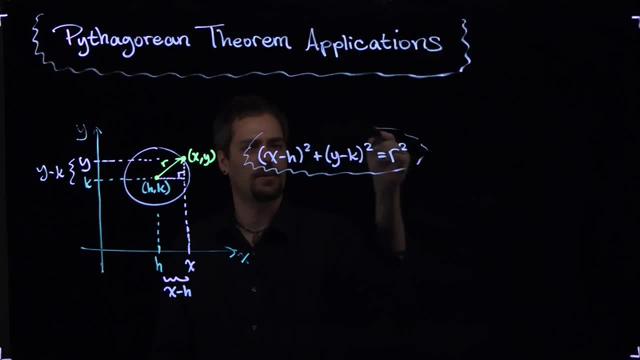 And there we've got what we call an equation of the circle. equation of the circle. Now, if you want to use it to have a y, let's say, on one side of the equation and x on the other side of the equation, then let's start by 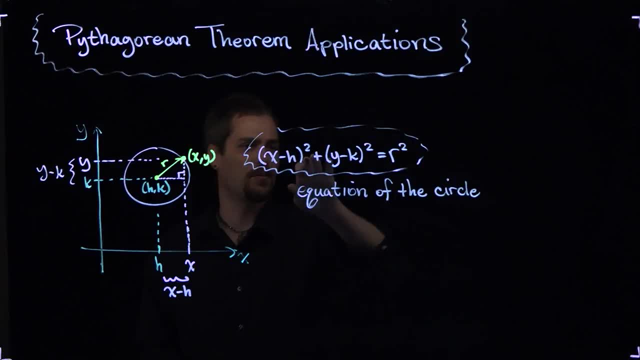 By getting this big chunk x minus h quantity squared over to that side. So just subtract it from both sides. That would give us y minus k quantity squared equal to r squared minus the quantity x minus h squared like. so Just subtract this from both sides. 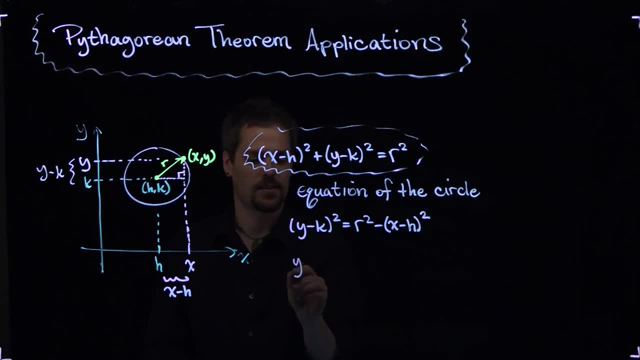 I could take a square root to get rid of that little square. Square root of both sides gives me y minus k equals plus and minus. the root of r squared minus quantity, x minus h squared- Very squeaky. And then I can add the k to both sides of the equation to get y in terms of everything. 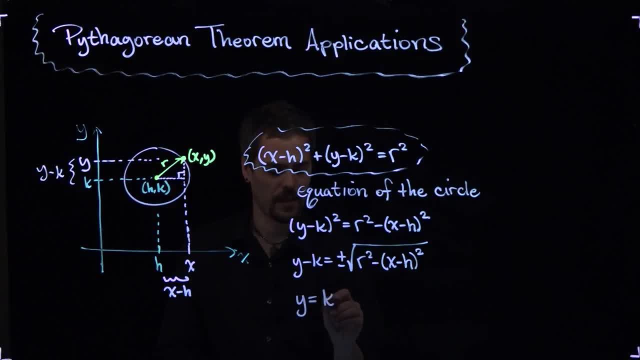 else. on the other side, Y equals k plus or minus square root of r squared minus the quantity x minus h squared. So there's another version of it where you have y in terms of everything else. This is one where, if you knew your hk, you knew where you wanted to start the center. 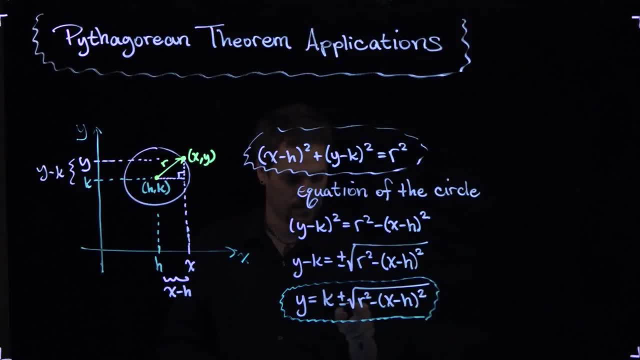 the center of it and you knew your radius over here. excuse me, you could stick that into a graphing application or just do it by hand and come up with a bunch of points. that creates this circle. Now you do have to be careful, because you've got one for the positive root and one for